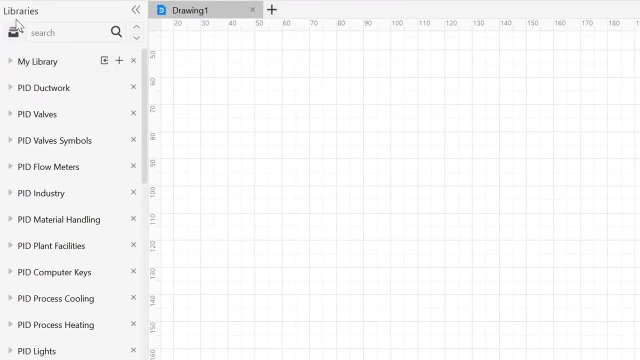 on the left side you find a library. In this library you can find all kinds of P&ID symbols like ductwork, valves, flow meters, industry material handling plant facilities, computer keys, process cooling, process heating. You can also create your own custom symbol by simply. 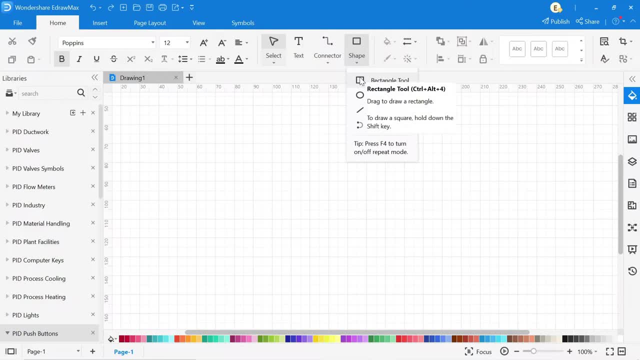 clicking on the shape. Here, different shapes are available. So select the symbol according to your drawing and draw your own custom symbol Here. the system symbols are shown in the right-hand side. On the right-hand side you will find the system symbol. You can also create your own custom symbol After that. set the system. 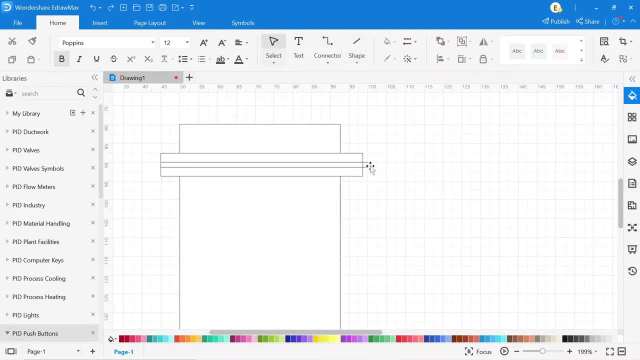 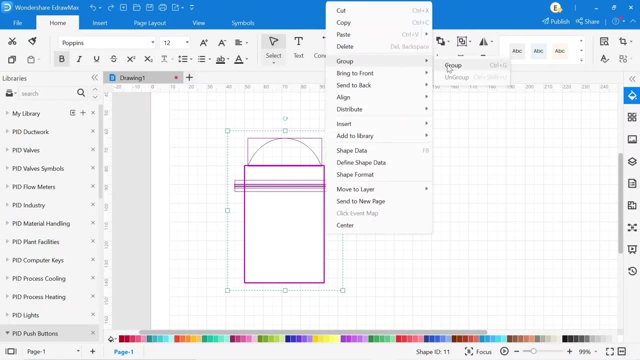 symbol as the system symbol. After that, select all and make them group and then click on the plus icon in the library. so the symbol will be added to the library. Here you can see that you can typically use the whole system symbol, but you can also 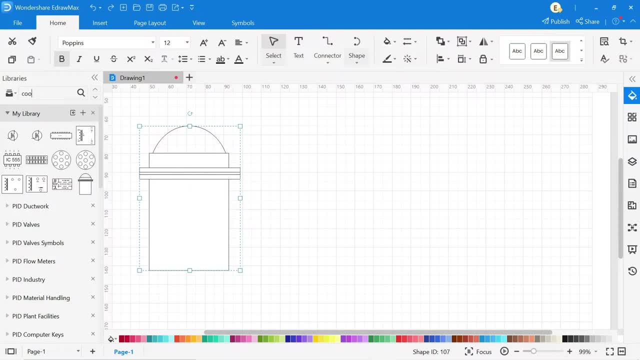 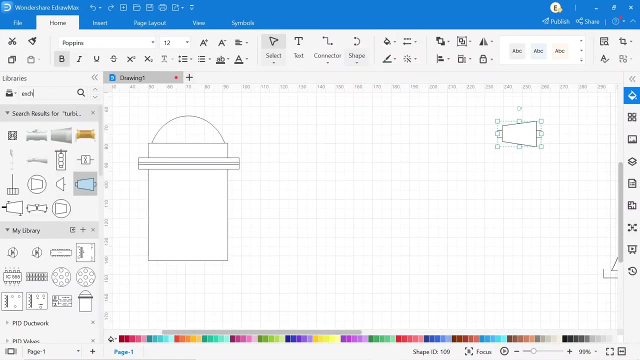 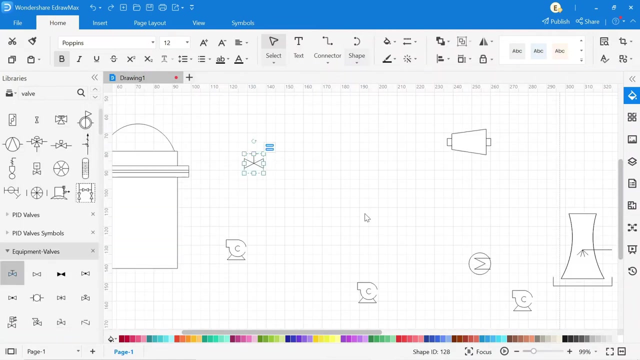 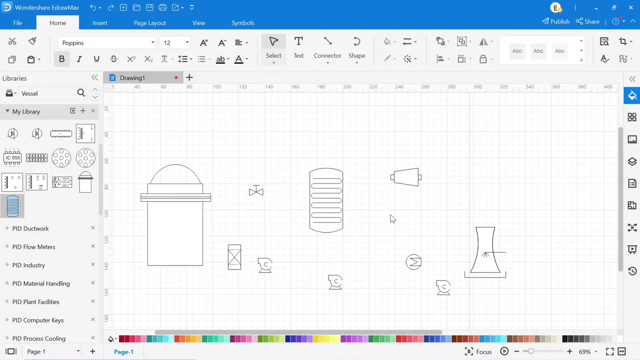 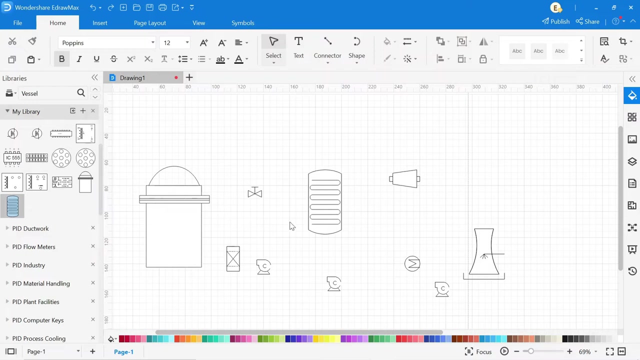 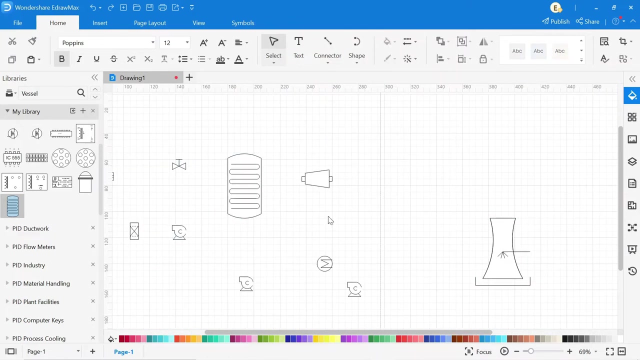 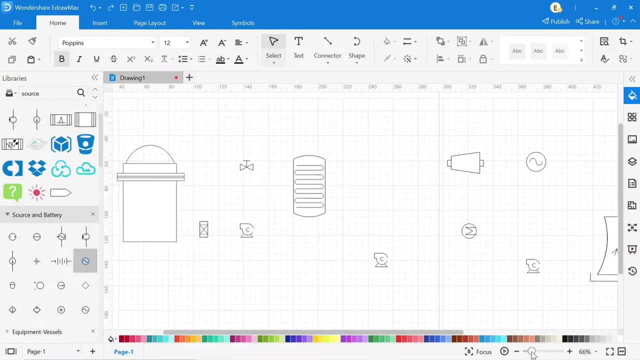 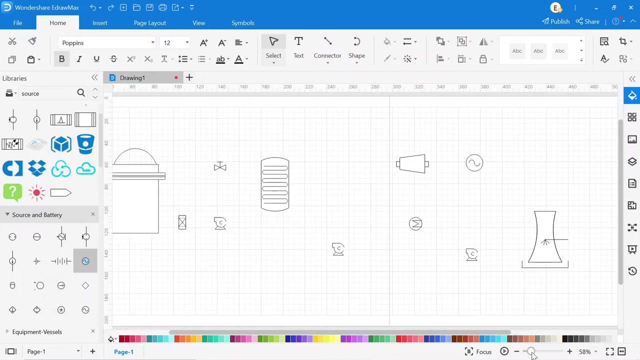 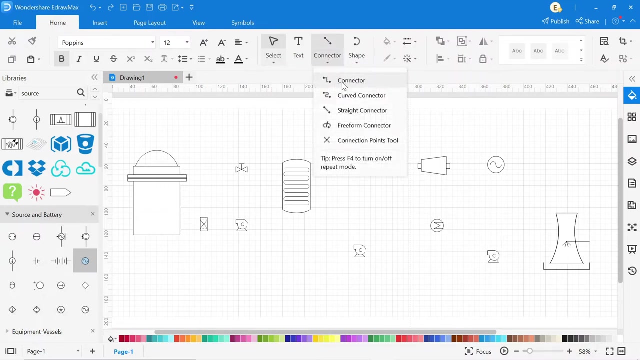 adjust the system symbol using another method. Here, for example, you can use a custom symbol. Now drag and drop all symbols according to your drawing To make a connection. go to the connector. Here different connectors are available, so select the connector according to your drawing. 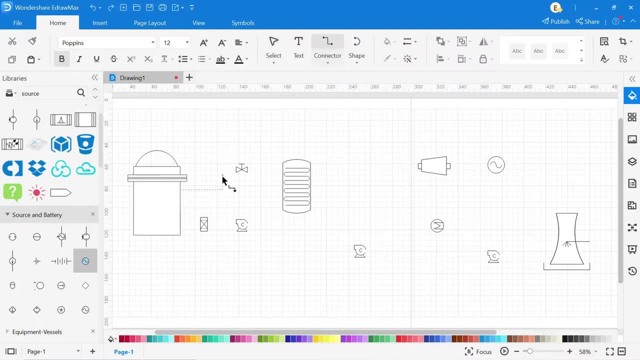 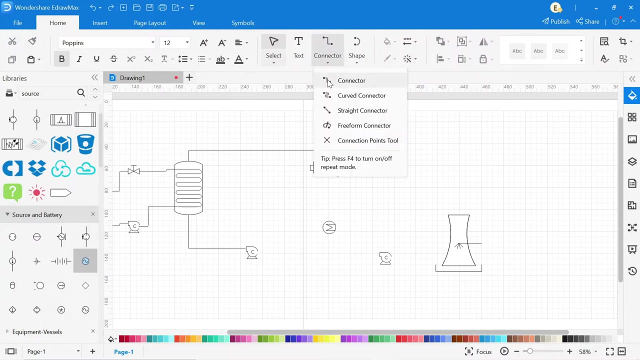 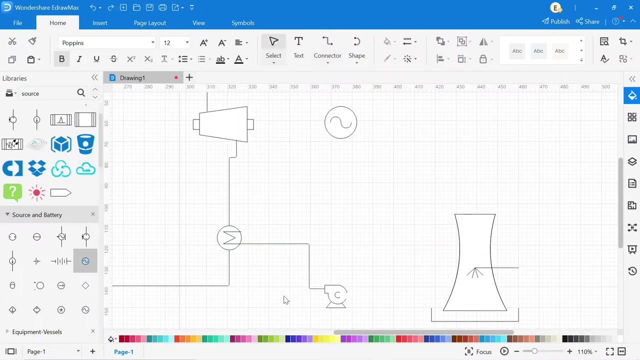 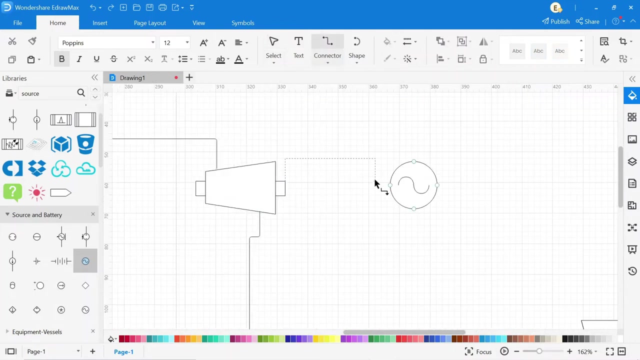 After that, select the connector. Simply draw all connections as per the circuit diagram. To make a connection go to the connector. Here different connectors are available, so select the connector. Simply draw all connections as per the circuit diagram. Here different connectors are available, so select the connector. 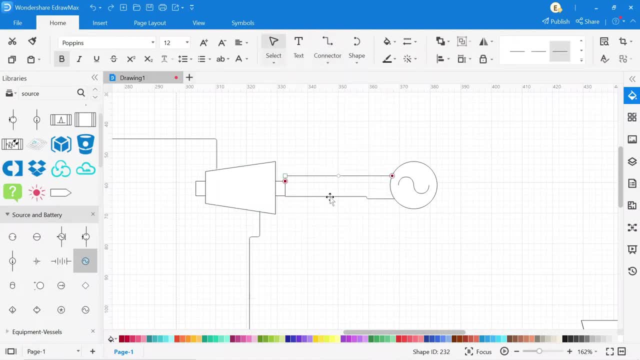 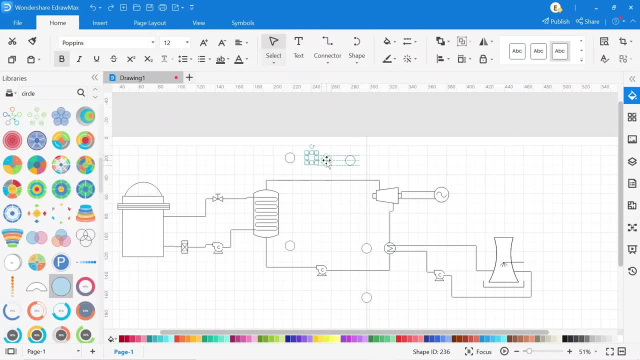 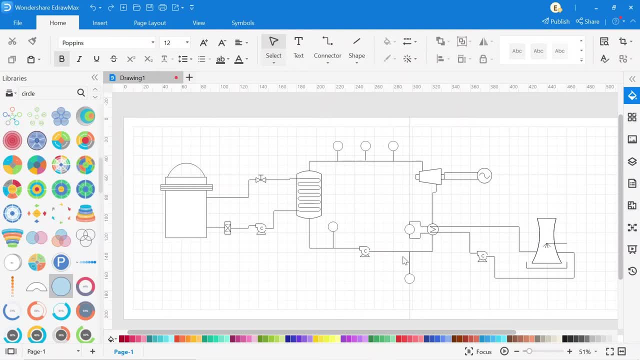 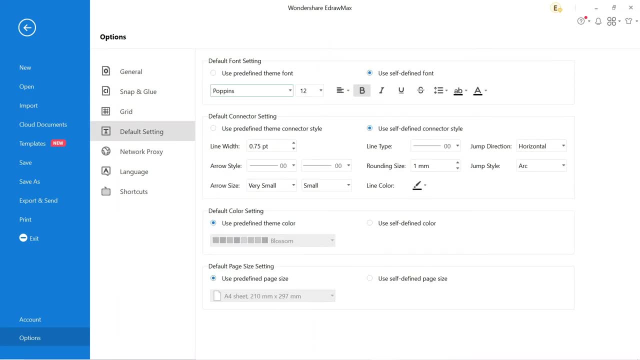 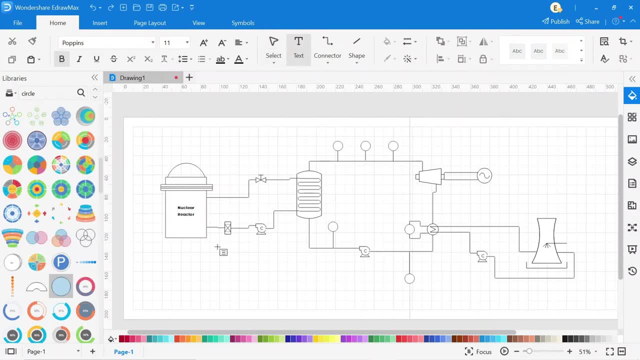 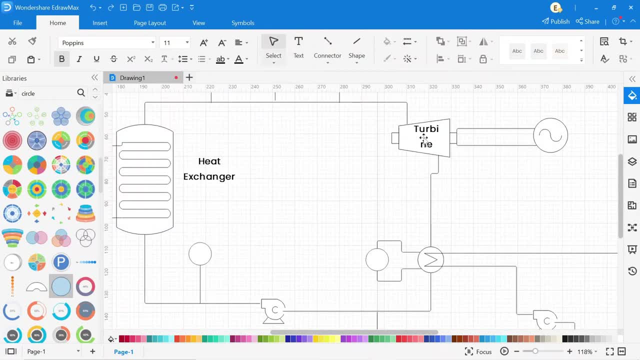 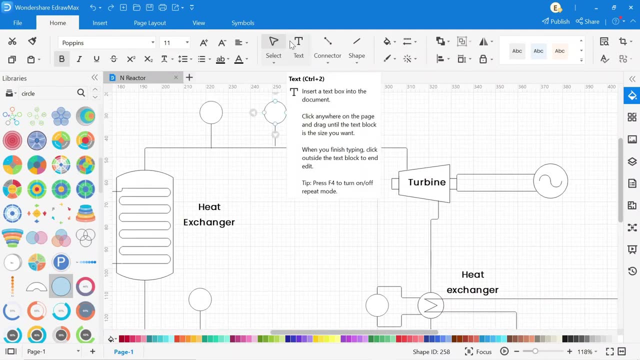 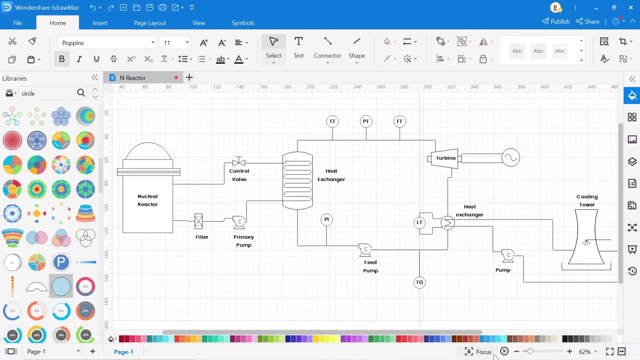 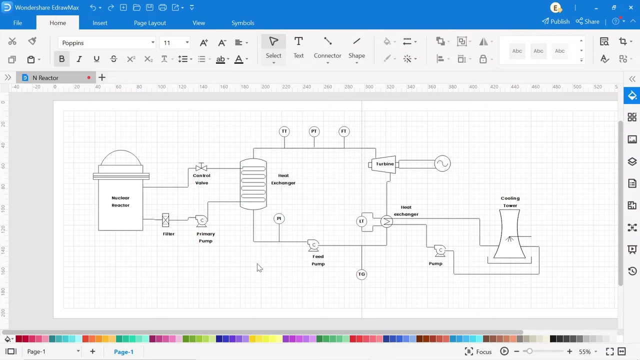 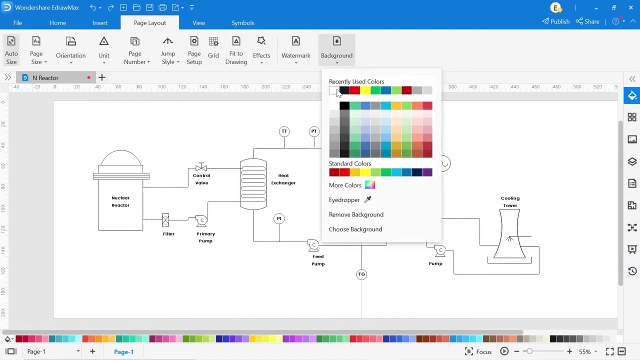 Here different connectors are available, so select the connector. Now our drawing is completed. You can also change the background color by simply clicking on the page layout. Then click on the background and select the background color you want. Then right click on the mouse, then click on the fit to drawing. 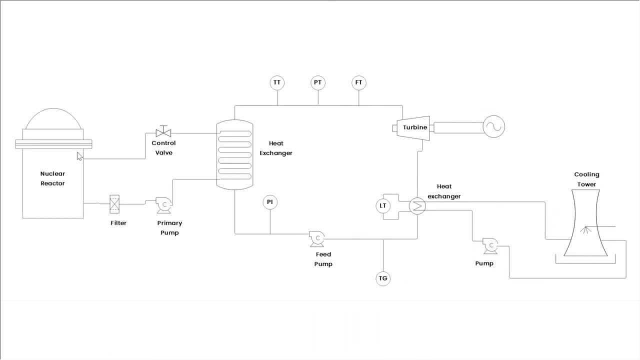 Here. first of all, heat comes from the nuclear reactor to the heat exchanger. In heat exchanger, water turn into a hot steam and then it goes to the turbine and due to high pressure of hot steam it rotates the turbine and electricity produced. 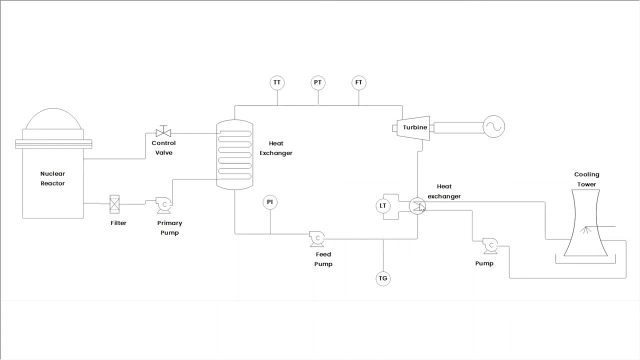 After that, vapor goes to the heat exchanger. in the heat exchanger heat is extracted from the hot steam and the cooling tower helps to extract the heat from the steam. and then it turns into liquid and goes to the pump, and from pump it again goes to the heat exchanger.